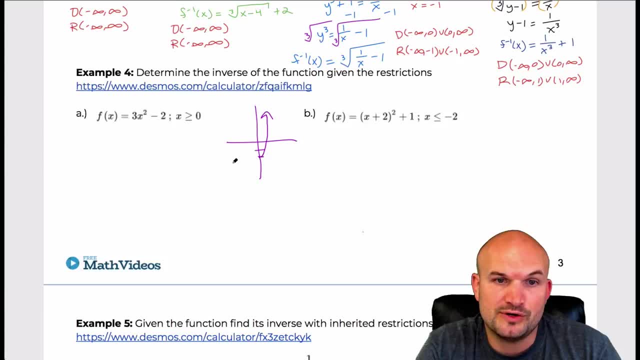 about the positive values of that function. So if we were to look into the graph of this, if I just wanted to kind of sketch this, I know the graph here is going to, you know, look, or should probably be like that. The graph is going to look something like that as far as the inverse graph, But let's 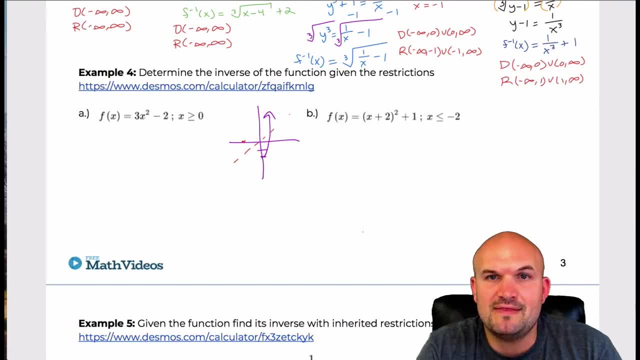 go on algebraically, go and figure out what the inverse graph looks like, And then you know, we can kind of compare our answers here. So again, following like really the same process that we've done before here, we're going to swap this for y and then we're going to swap the variables. So 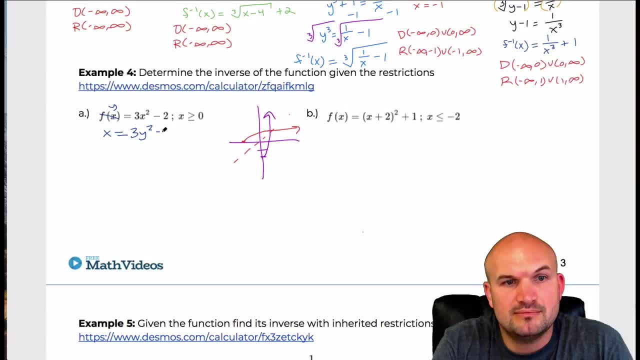 we have: x equals three, y squared minus two. Okay, And now to solve for y, I need to use my inverse operation, So I'll add a two. actually, let's zoom in here, So I'll add a two on both sides. 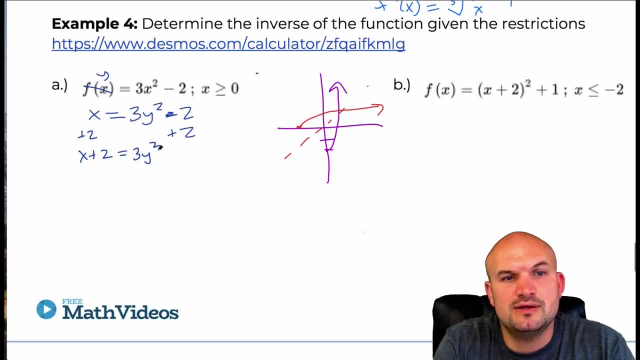 So therefore, I have x plus two equals three y squared divided by three, divided by three on both sides. Again, I prefer to use the inverse operation, So I'm going to add a two on both sides. I prefer to write instead of dividing by three, I prefer to write this as a one third in front. So 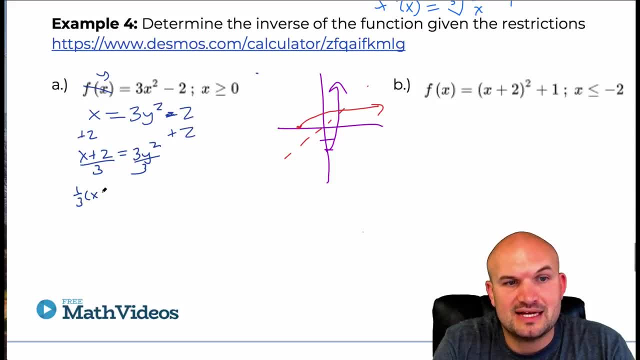 therefore, I can rewrite this as a one third times x plus two. Now you could distribute that three into both of them, but I'm going to show you and explain why that is not a preferred method in this case. So here we have y squared. Now again to get rid of the squaring we're now going to need. 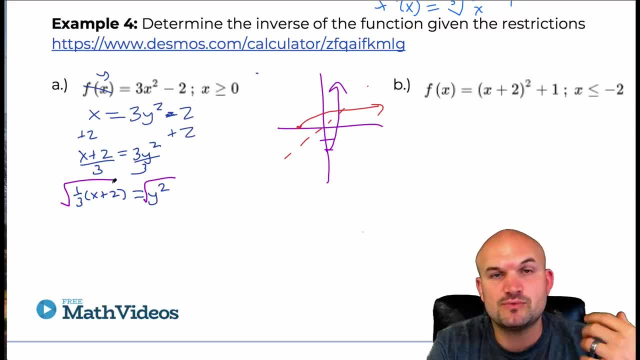 to take the square root of both sides, And this is where it becomes important. This is where it's different than the cubic root, because the square root, as a restriction, it has that implied restriction. We can't take the square root of a negative. 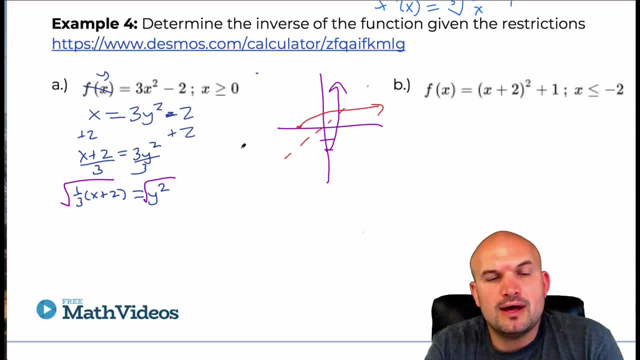 value. But in this case, since our original function was since this and again, hold on, let me get to that point. You can't take the negative root. So that's one part of our restriction. But then the other thing is: when you introduce the square root, you have to include the plus or the 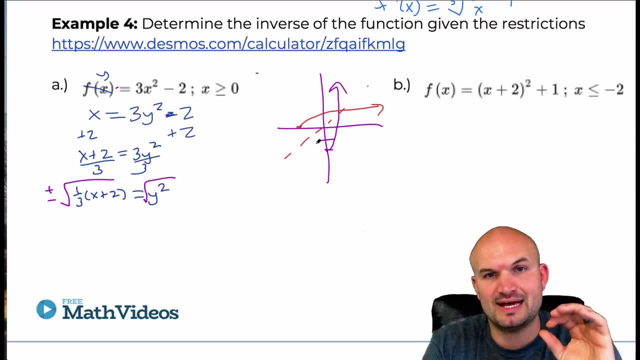 minus. And what that makes us happen, or what that allows us to do, is now we have two solutions. Now when we solve for y, which is really going to be our f inverse. So now when I say, you know, f inverse of x, I have plus or minus the square root of one third x plus two, And but fortunately for 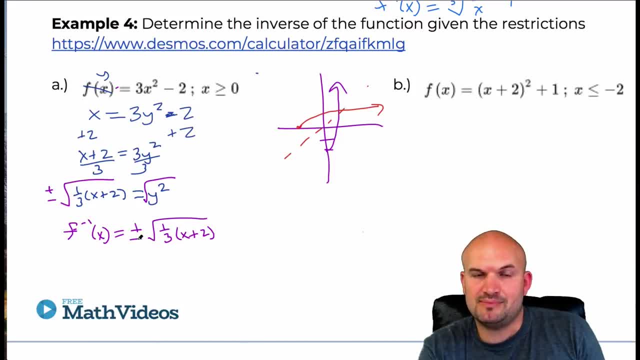 us. we. that's not going to produce a function right, Because you're going to have, for every x value, you have two y values. So that's definition of function doesn't work. But since we have this restriction where my x values are going to remain positive, I'm only going to include the positive. 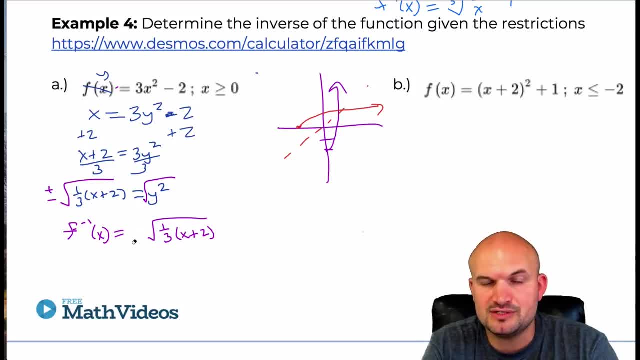 root. Now I don't need to write plus square root, I can just delete both of those. but we just know. now we're only going to inquire about the positive root of of our inverse function. Now the next thing: the reason why I'm keeping this as one third times x plus two, is because this tells us: 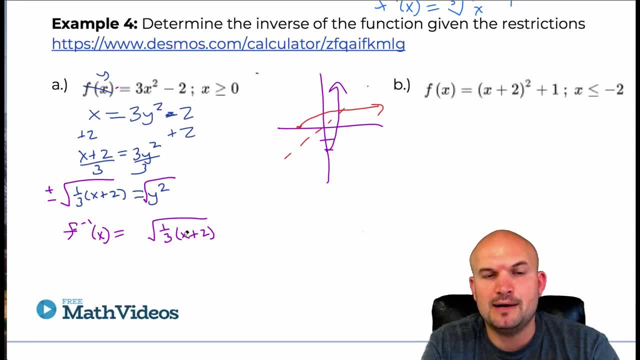 what our transformations are. If you remember our previous unit of transformations, this is in the form of b times x minus c, right? So this plus two is telling me to shift the graph two units to the third. What that's telling me is that's going to be a. the one third is telling me that's going to. 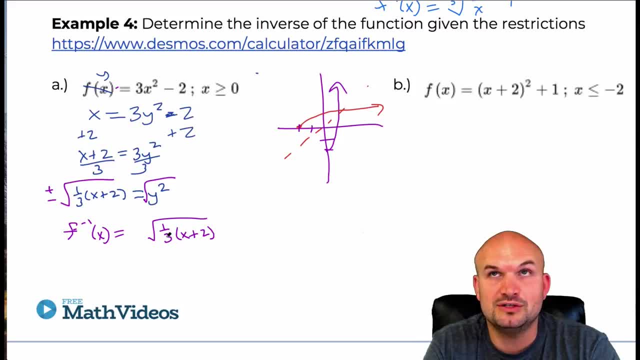 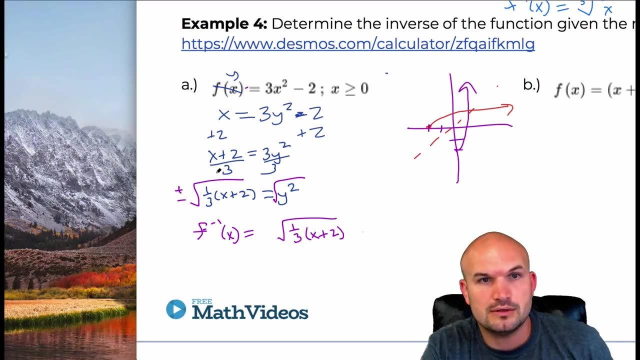 be a- let's see, that is going to be a vertical stretch or, I'm sorry, horizontal compression of that form too. No, Yes, I'm like mixing up my things. Let's go and take a look at the graphs and my thing will come back up to me. Oh no, Why do you do that to me? All right, I don't know why. 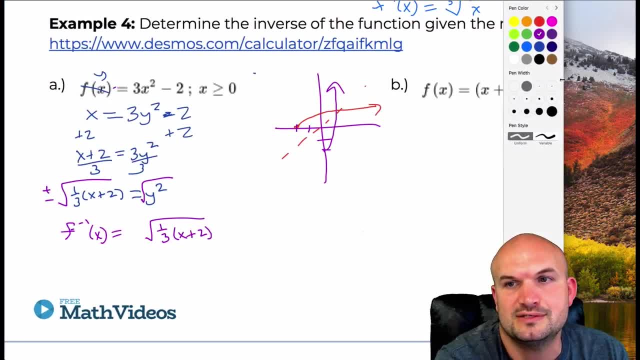 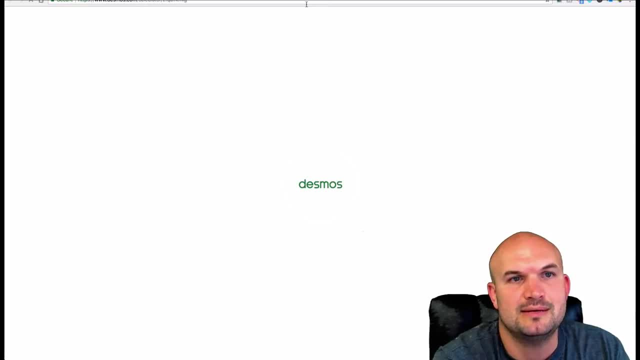 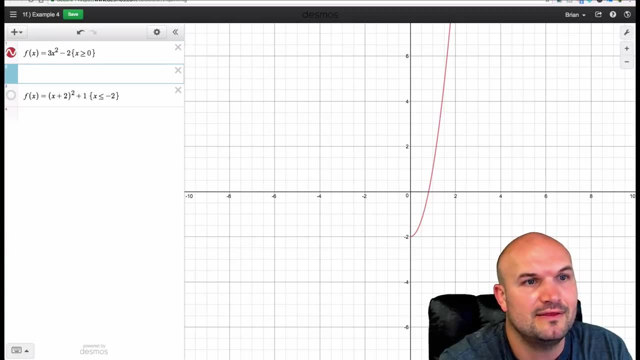 that happens. So let me just go and fix this, All right, So I'll bring it back up in here. Let's go in and look at example number four. Oh, so there's exactly what the example looks like. And then let's go and see what the inverse function, So that's f of x, equals the square. 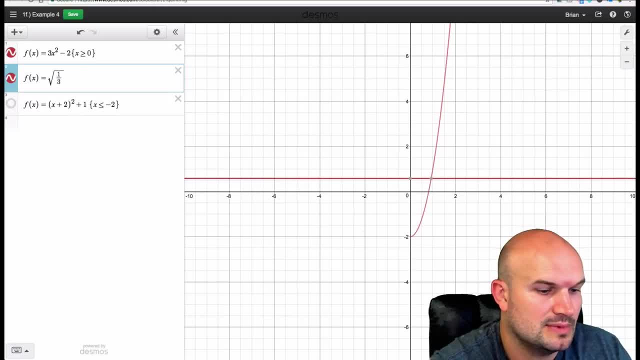 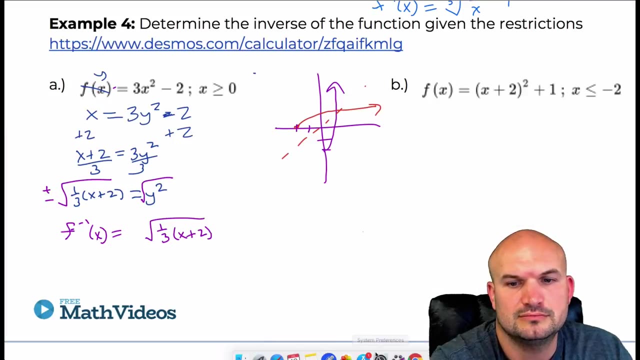 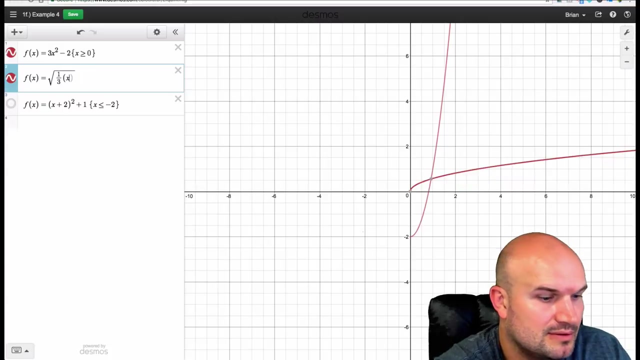 root of one divided by three. And then that was times um x. I forgot what- the x minus two. So x minus two. Oops, That's plus two. I'm sorry, The inverse was x plus two And therefore you can see that. yes, that is the inverse function. 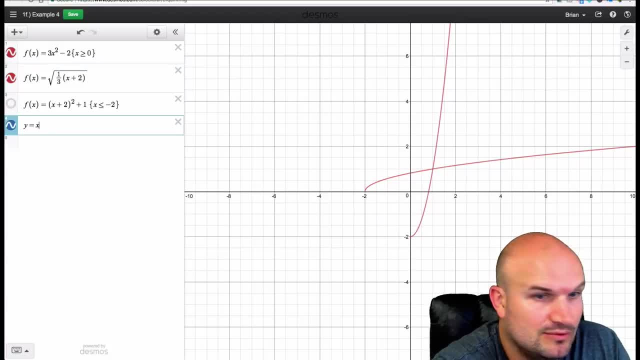 That is now reflective about the equation y equals x, right, So you can see how those uh now work. So that's very, very important. It's of our horizontal stretch, Yeah, Cause that's same thing as vertical compression, So it's a horizontal um that one third. Yeah, It's a. 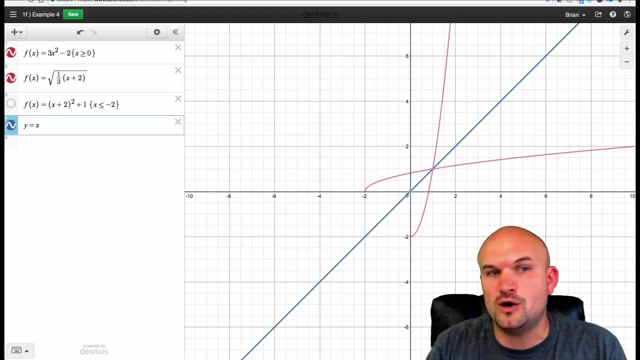 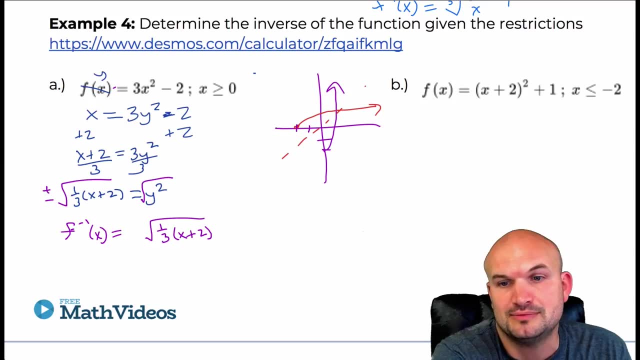 horizontal stretch. Um, so there we go. there You can see how that works by restricting that domain, because if I didn't have that domain restriction, I wouldn't have a function, I would have a sideways, uh, parabola. All right, So let's go and work on the next example here, And then we'll. 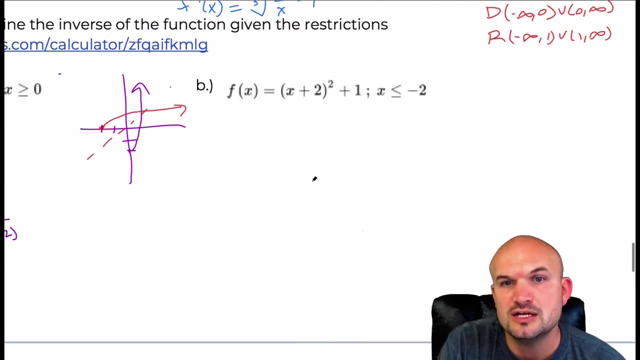 go back to Desmos to kind of verify our result. So in this example we have another function, or we have another quadratic, and this one is in vertex form. All right, Um, and we have a restriction now for x values that are less than or equal to negative two, And again we have enough. 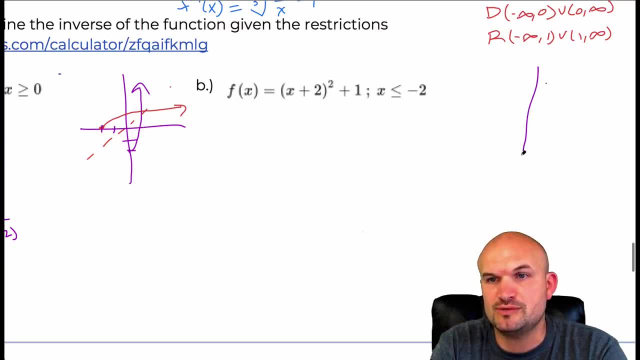 information right now, to kind of graph the quadratic with the restriction, without the restriction. So let's just go and graph it and then we can verify. on Desmos, So this has been, uh, shifted: two units to the left and one unit up, and a is one positive one. So it's going to be a. 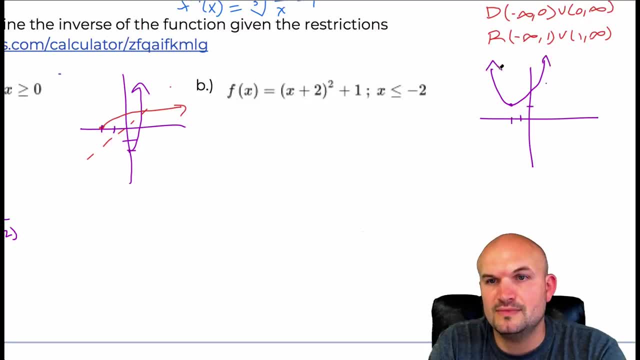 nice little quadratic here. It's going to look something like that, Right? But again, my restriction is going to be less than or equal to negative two, And again we have enough information on this. my restricted domain here is only values that are less than negative two, So therefore I can. 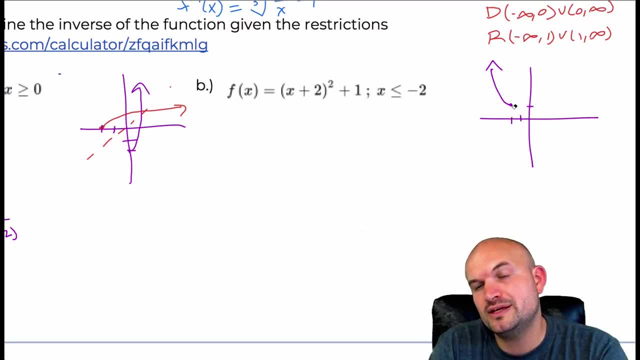 just simply delete that portion. I'm only going to be finding the inverse of the for values of x that are less than negative two. All right, So now let's mathematically go ahead and find the inverse. So we'll replace this with y. swap the variables So x equals y plus two squared plus. 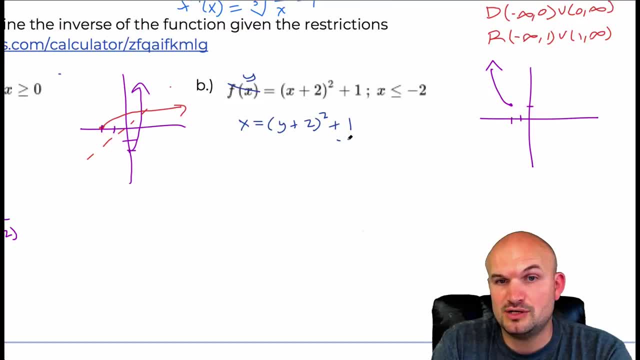 one. Now what we want to do is again go ahead and solve for y, So I'll subtract a one on both sides. So I get x minus one equals y plus two squared. And now, geez, come on. 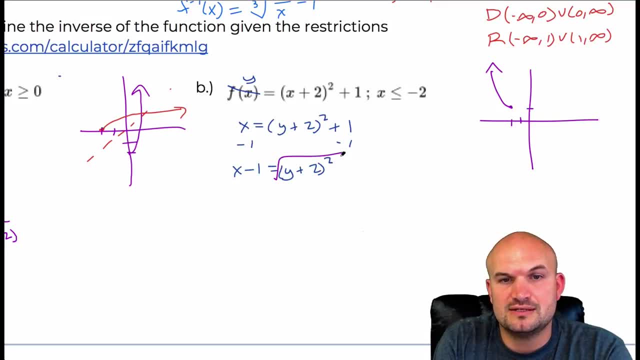 Now I'll take the square root of both sides, So we'll root both sides. Now again, when you introduce the square root, you have that plus or minus, right? Um? so therefore I have you know, y plus two equals plus or minus the square root. 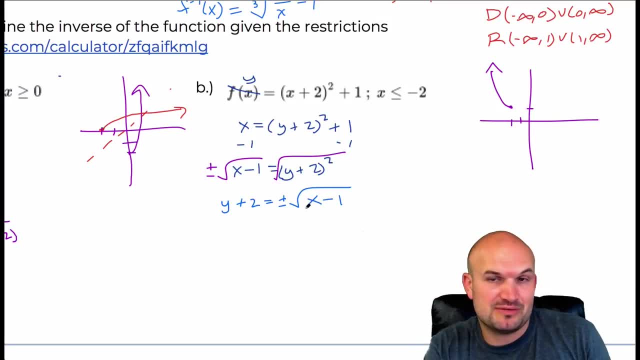 Of x minus one. But again, we don't want to be dealing with the plus or minus because that's not going to produce a function. So we've got to determine: is it going to be the positive or is this going to be the negative? And you can see that our restriction is going to be, you know. 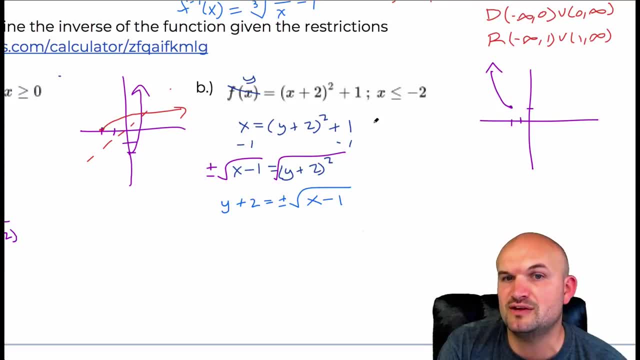 to the left, the more negative values of that vertex. So therefore we're going to want to include in this case the negative root and we'll see why that's going to work, or why that's going to help us justify here via Desmos, And then we'll subtract two on both sides and we get a final. 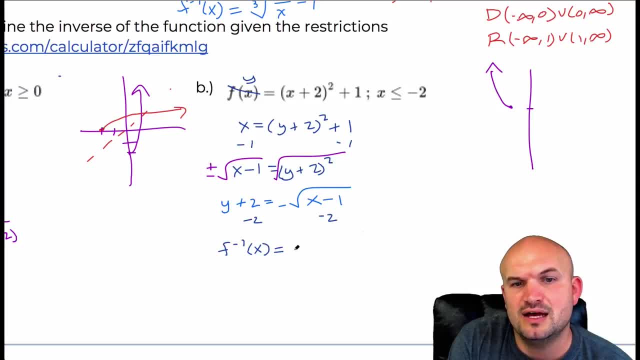 uh inverse function and f- negative, negative x of negative square root of x minus one, minus two. So if we were to graph that, I don't know what happened here. So that's left two. So if we were to graph this, all right. so this is a radical function that has been reflected. about the x: 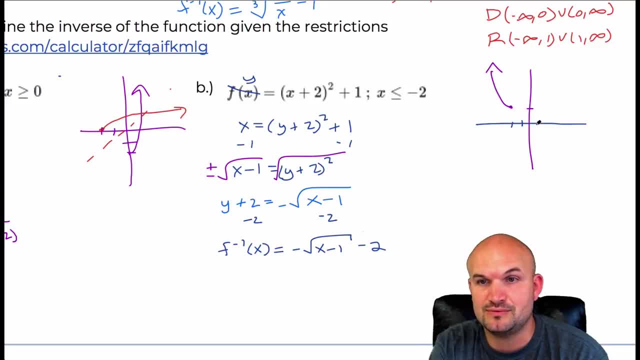 axis. It's being shifted one unit to the right and down two, So it's one, two And then you can see that it is reflected. So if it was not reflected, look like that, but sort of reflect about the x axis. It's going to look something like that, right? So let's go into uh, Desmos. 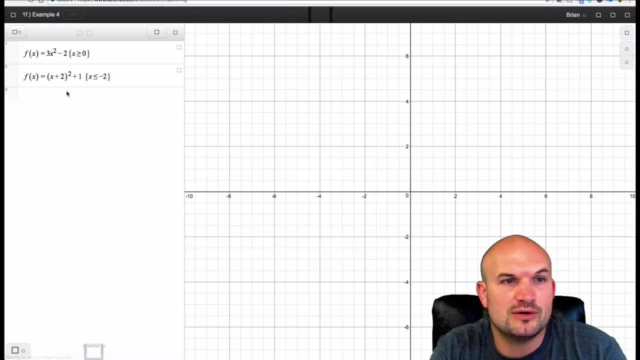 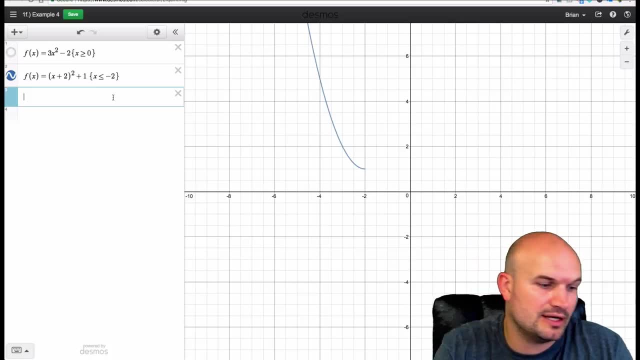 I guess we'll just go to the same browser here and just to confirm our result. There you go, And then, if I go ahead and click on a new one. so f of x equals, let's say, negative square root of x minus one, minus two. 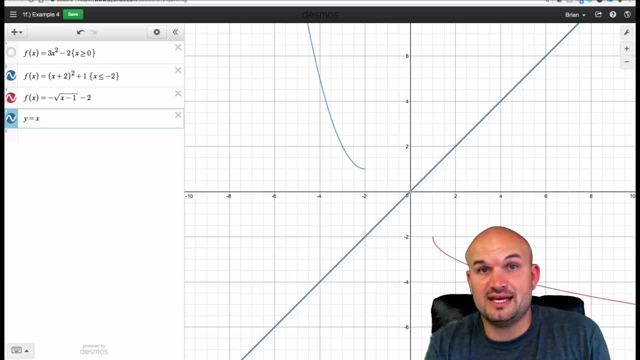 And then let's plug in the y equals x line And you can see that they are symmetrical, right? So I did my work. um, you know, correct? but it's very important to understand how those restrictions, when they are provided to us, are going to play a part in, uh, writing the domain. 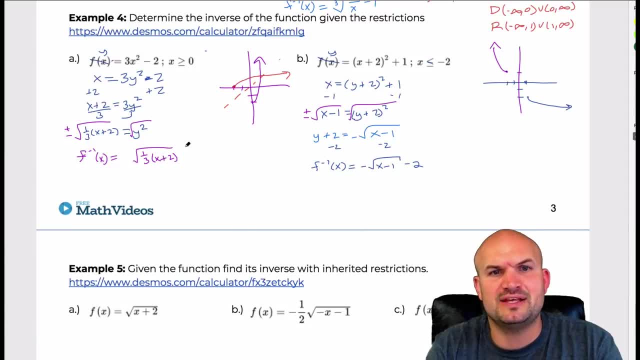 I'm sorry, not even writing the domain, but understanding uh the function, as well as understanding the uh uh the function and its restriction. Now it's also important We are restricting the domain here, right? So if we're restricting the domain, guess what that tells us? that automatically tells us the range of. 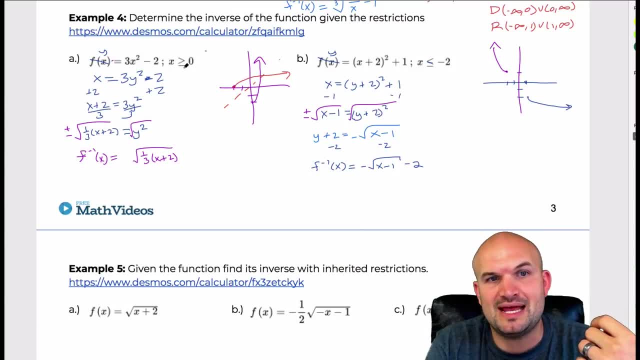 our inverse function. right, I don't even need to think about this. If I know, the domain of this purple graph is greater than zero. well, that means the range of my function is going to be for y values that are greater than zero. Think about this one: x values are less than negative.